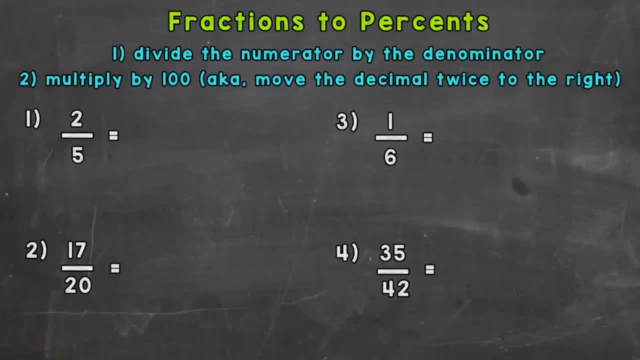 Numbers two, three and four. I'll give you the answer that you'll get if you punch these in on a calculator and how to put that into percent form. So again, here we have two, Two fifths. So we need to divide the numerator, or top number, by the denominator. 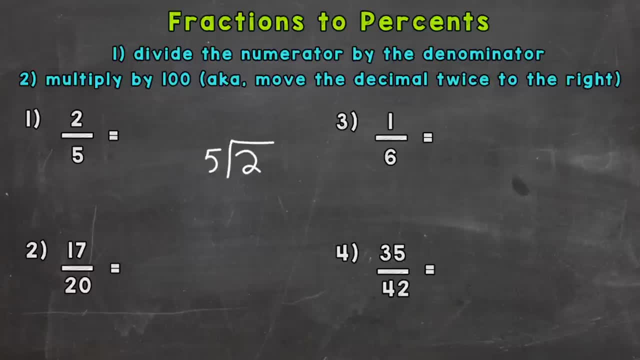 So two divided by five. We cannot pull a whole group of five out of two, so we need to extend with a decimal and a zero. Now bring the decimal straight up and we have 20 divided by five. So how many whole groups of five out of 20?? 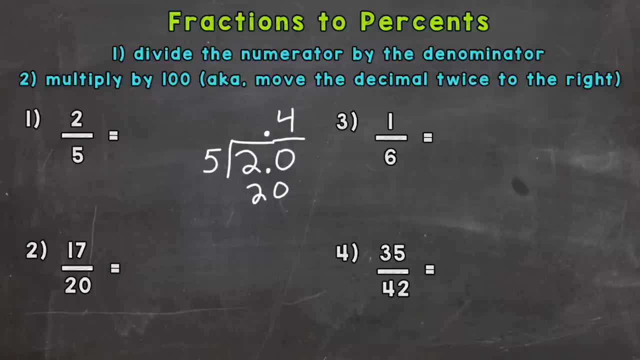 Well, four, Four times five. Four times five is 20.. Subtract: we get zero. So our answer for step one, dividing the numerator by the denominator, is four tenths. Now we need to multiply by a hundred, and we can do that by moving the decimal twice to the right. 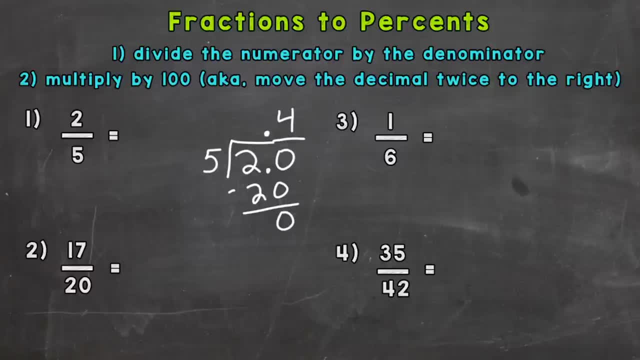 And the reason we multiply by 100 is because percent actually means per 100. So multiplying that answer gives us that per 100. Which is the percent. So let's move. I'm going to rewrite four tenths down here and move the decimal twice to the right. 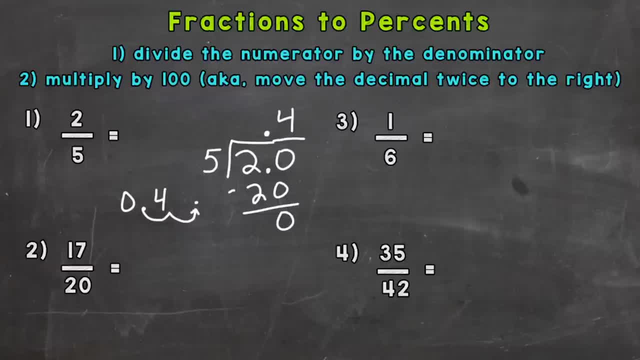 One, two Fill with a zero here, and we get an answer of 40. Which in percent form, 40 percent. So two fifths equals 40 percent. Number two: 17 twentieths. Number two: 17 twentieths. 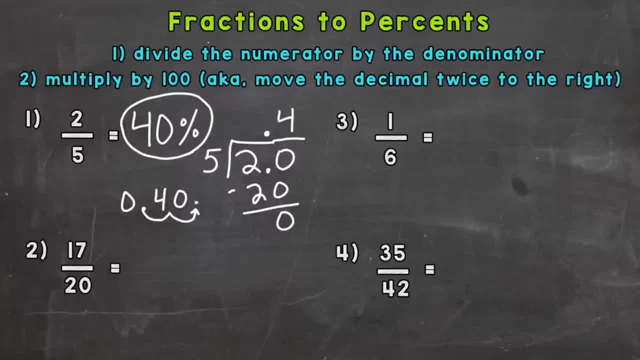 Number two: 17 twentieths. So 17 divided by 20 gives us 85 hundredths. So that's step one, Step two. multiply by a hundred, Move the decimal twice to the right One, two. So the decimal is now at the end. 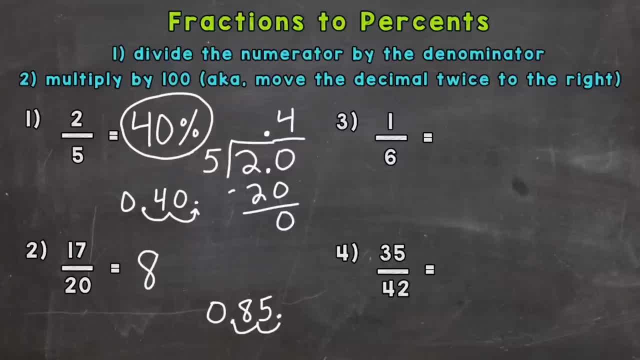 17 twentieths equals 85 percent. Number three: we have one sixth, And this one's a unique problem because we get a repeating decimal. when we divide one by six, We get an answer of one, and then six is repeating. So they go on forever that way. 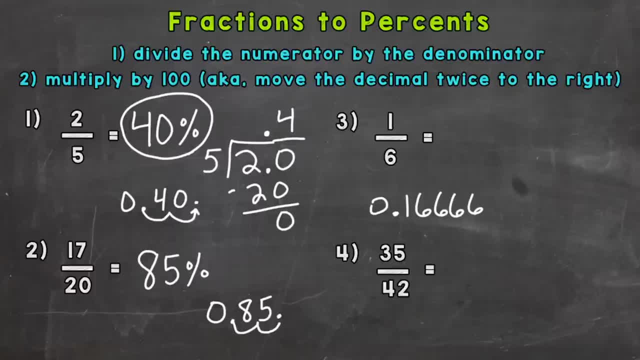 But we follow the same steps. It's just how you want to represent your answer. So let's multiply by a hundred, Move the decimal twice And we get 16.. 16. And six is repeating. So we can put a bar above that six to show it repeats. 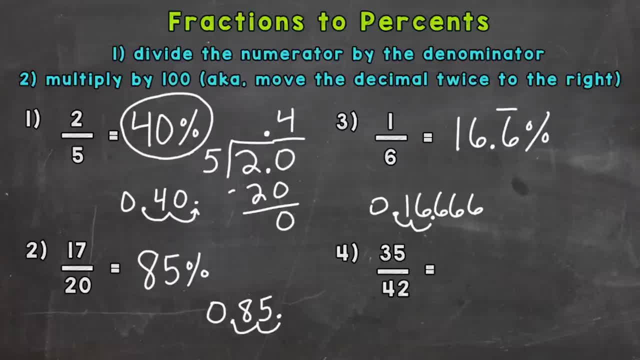 And that is percent. Now you can also round to represent that answer. You can round to the nearest whole percentage, Tenths, hundredths. So for example, the nearest whole percentage would be 17 percent, 17 percent, 17 percent if we rounded. 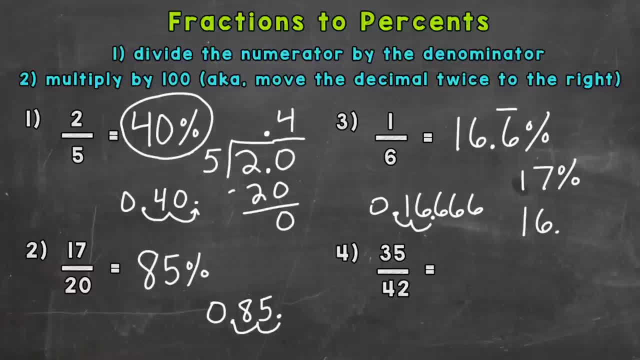 Or tenths place would be 16 and seven tenths percent. So again on the repeating decimal percentages, same steps. You just have to determine how you want to represent that answer. Number four is another repeating decimal. We get eight and then three's repeating. 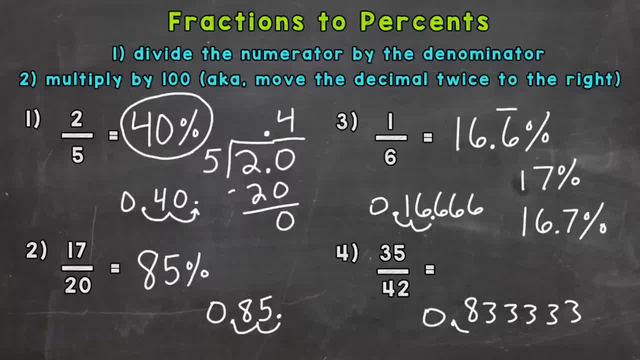 So again same steps. Multiply by 100.. Move the decimal twice And we get 83 and three's repeating percent. Or if we rounded to the nearest whole percentage, this would be 83 percent, Or tenths would be 83.. 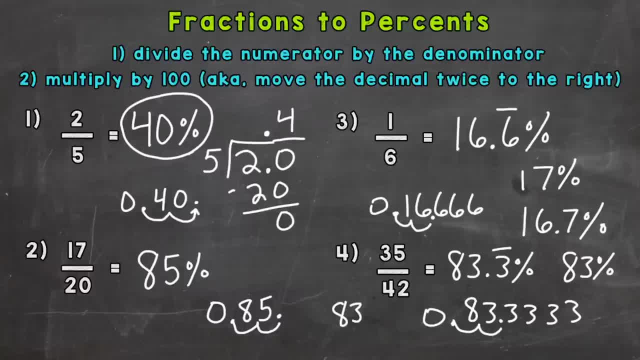 I'll put it over here, to the left, running out of room 83 and three tenths percent. There you have it. There's how you go from fractions to percents. Divide the numerator by the denominator And then multiply by 100.. 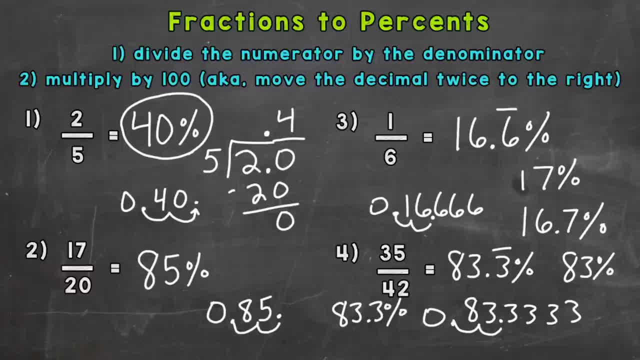 Because remember, percent means per 100.. Hopefully that helped. Thanks so much for watching. Until next time, peace. 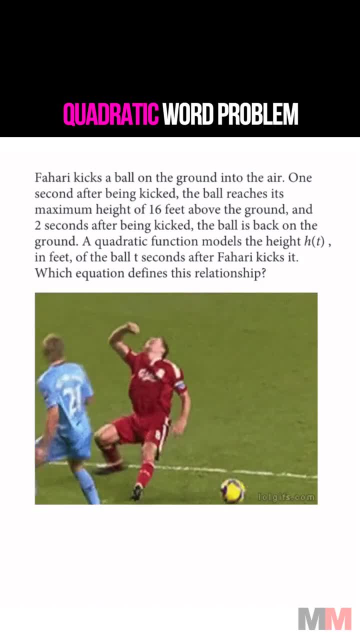 a heart kicks a ball on the ground into the air. one second after being kicked, the ball reaches its maximum height of 16 feet, and two seconds after it being kicked, the ball is back on the ground. which equation matches that scenario? a ball is kicked on the ground, so we start at zero.